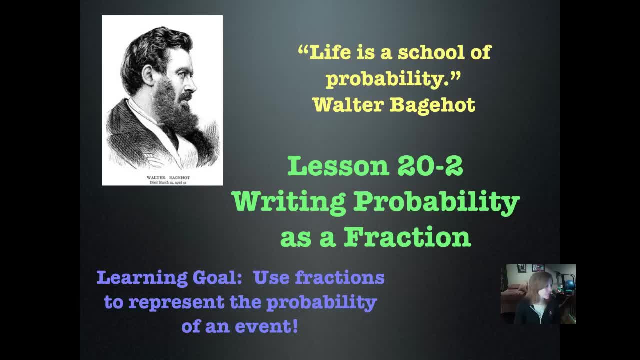 and he wrote about politics and the economy and government stuff too, and literature. So I had to look him up. I didn't know anything about him and when I read his quote- which I liked because it's about probability- I had to learn a little bit more to be able to share things with you. 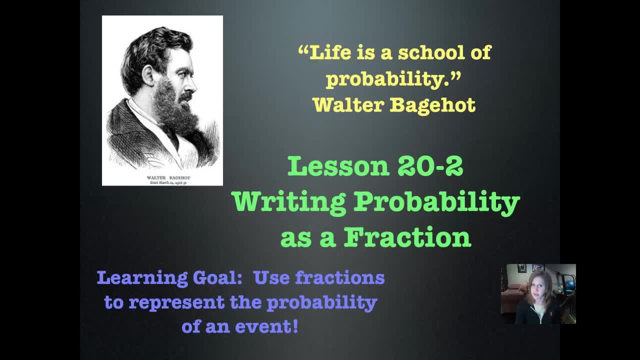 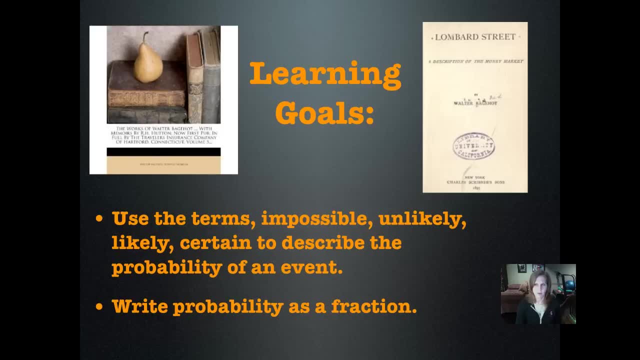 Our learning goal tonight is to use fractions to represent the probability of an event. There are some books that he wrote Lombard Street Description of the Money Market and that does. That copy belonged to the University of California. Kind of cool. 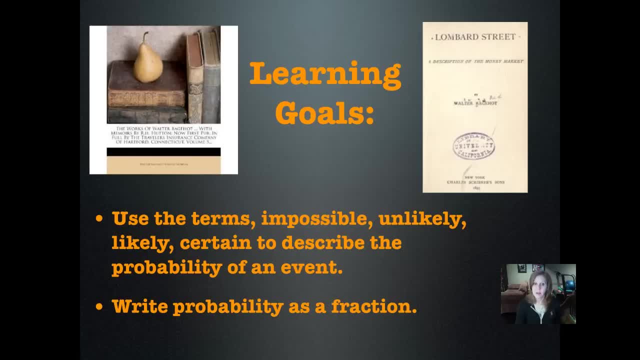 Here is our individual lesson learning goals. Use the terms impossible, unlikely, likely and certain to describe the probability that an event will occur, And we're going to write probability as a fraction and use those fractions to decide which terms to use. Here's our vocabulary. 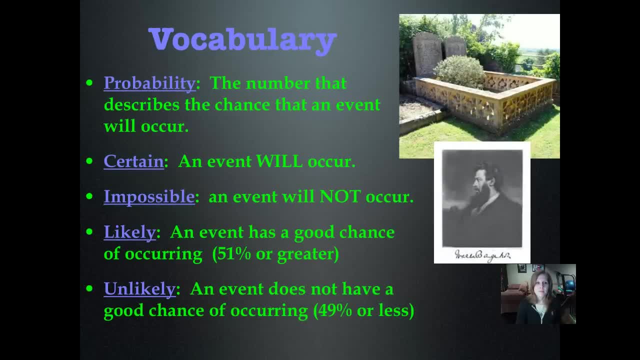 There's his grave. It's kind of fancy looking Probability. It means it's the number that describes the chance that an event will occur. So if I asked you, what is the probability that you're going to have homework on a school night? 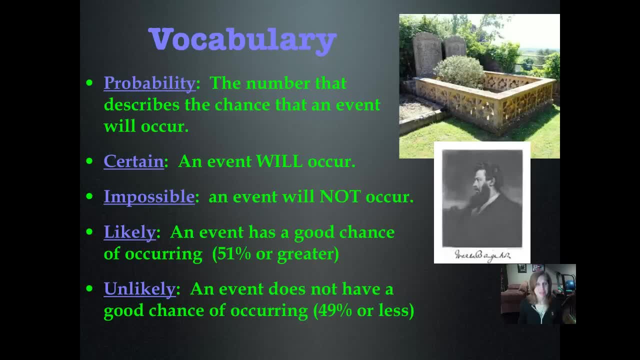 It would be likely, Absolutely likely. What would be the probability that you are going to have to be in fifth grade again? Unlikely, And we could probably almost go to impossible, because all of you have worked really hard this year. What is the probability that you will enjoy your math class? 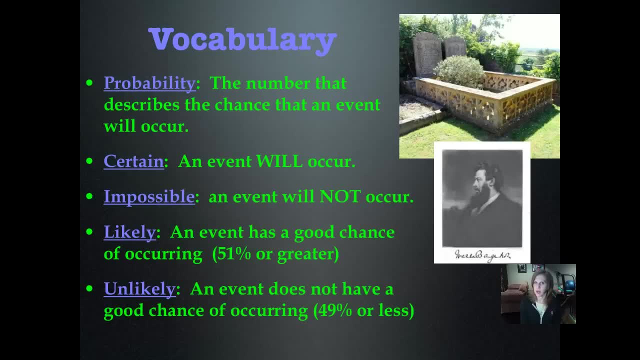 Hopefully Likely. What is the probability that I will give you homework on a Friday? I've done it a couple times, Maybe unlikely. I don't usually give you homework on a Friday. What is the probability that I am going to eat lunch? 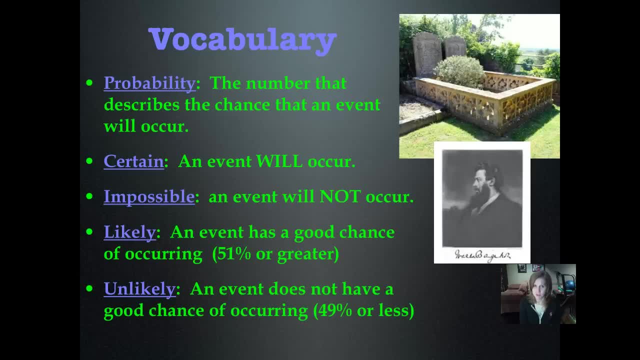 Certain, I never miss lunch, It would be certain. So all of those are just some different examples of the way we use the term probability. Sometimes we also use the term likelihood: What is the likelihood that I will eat lunch today, Certain? 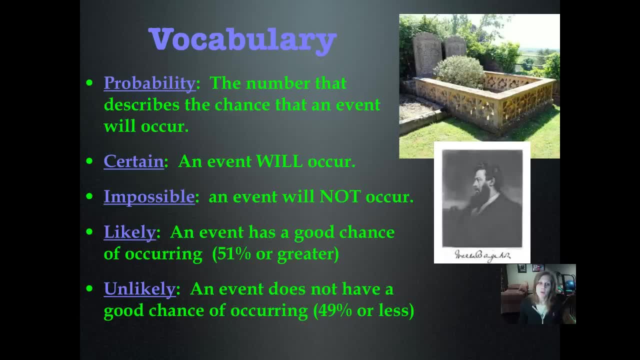 I will certainly eat lunch today. So there's our definitions of those words. Certain means an event will occur. There's no chance it won't occur. Impossible means an event will not occur. Under no circumstances will it happen. Likely means you have a 51% chance or greater that an event will occur. 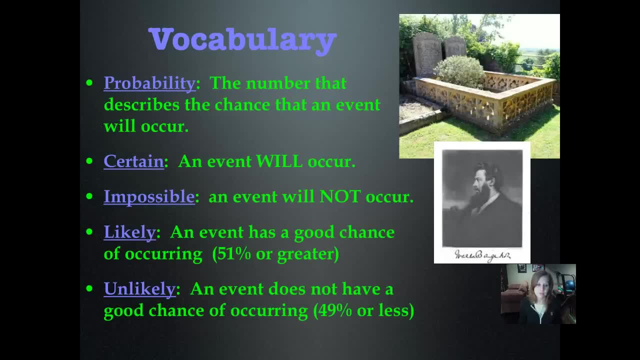 Remember, with fractions that would be greater than one half, Unlikely means you have a 49% or less chance that something will occur. That would be less than one half if you were using your fractions as probability. Let's go ahead and take a look at some of those. 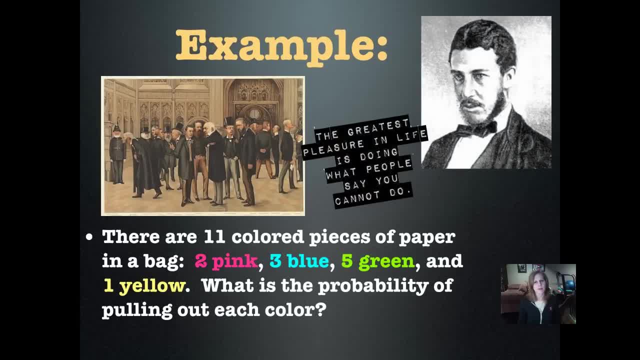 Here's an example. This is one of the things that Gadget said. He said The greatest pleasure in life is doing what people say you cannot do, And since he was a pretty conservative guy, you can see him standing in the middle of those groups of important men. 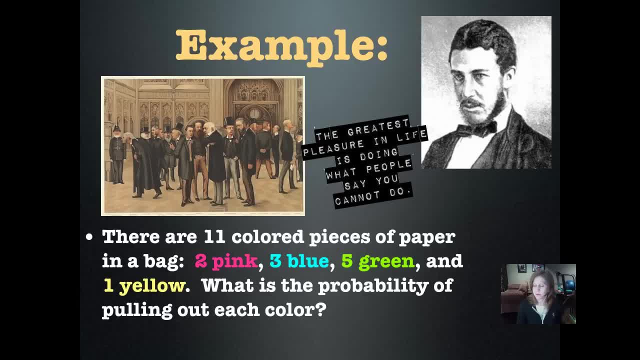 I don't think that he was saying that you should do things people tell you not to do. Like, if your teacher tells you not to talk in class, that doesn't mean you should get pleasure out of talking in class. I think it means that if people tell you math is too hard for you, 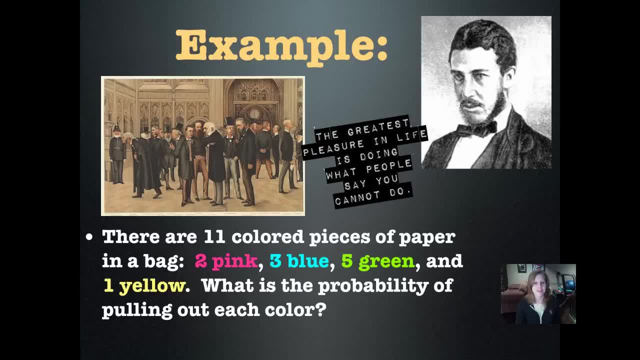 you should say: Hey, I get a lot of pleasure out of doing hard things that people say I can't do, And then just enjoy, Enjoy your success. Here's our example: There are 11 colored pieces of paper in a bag. 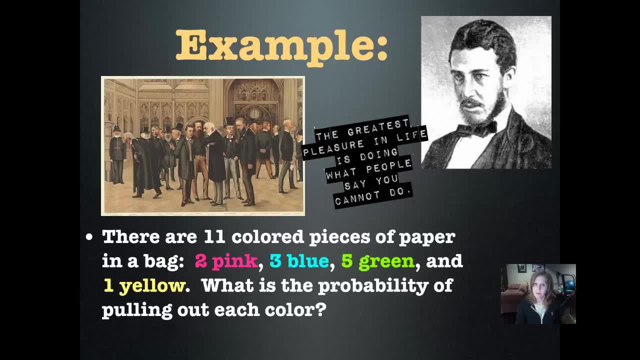 Two pink, three blue, five green and one yellow. What is the probability of pulling out each color? We're not only going to write the probability of pulling out each color in fractions, we're also going to use those terms we talked about earlier to describe the probability. 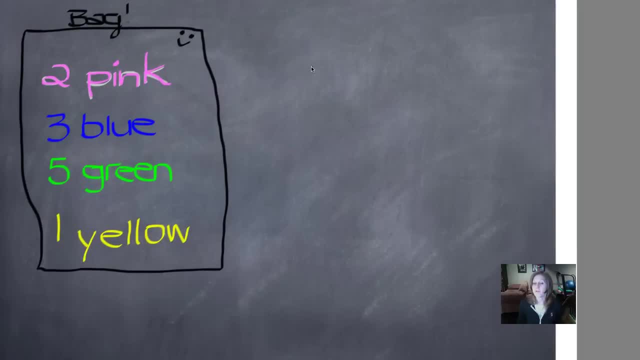 Let's do that now, Okay. So first of all, we have to know in order to write a fraction, because a fraction is always showing how much of a whole, So we need to know how many colored slips of paper we have in all. 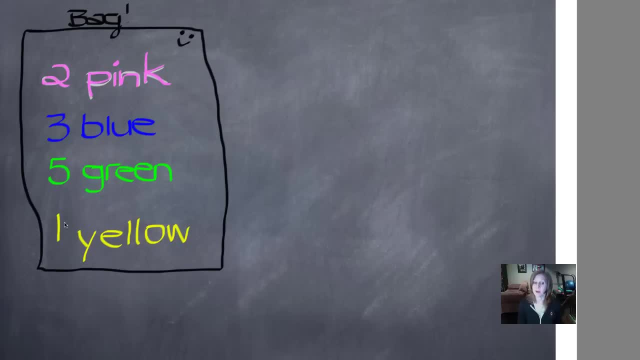 So here's our bag. We have two pink, three blue, five green and one yellow, So we just need to add those up. Two plus three is five, Five plus five is ten, And ten plus one is eleven. 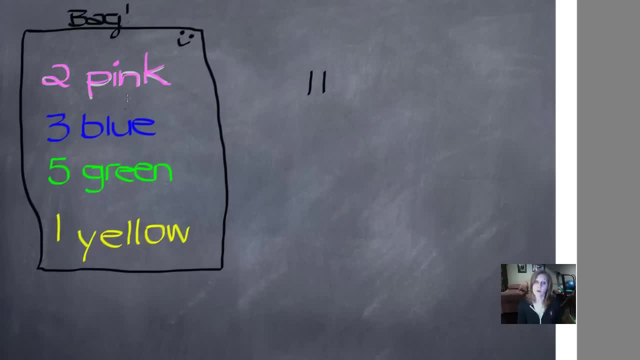 So eleven will be our denominator for each color. Now, if we're talking about pink, we have two pink slips of paper in this bag. So out of eleven slips of paper, there are two chances of us pulling out a pink piece of paper. 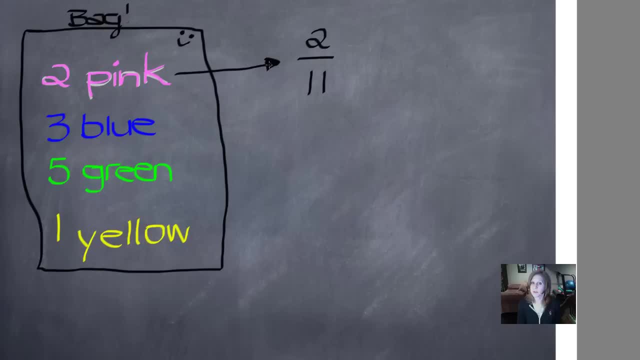 So the fraction that represents the pink pieces of paper is two elevenths. There are three blue pieces of paper. So there are three of eleven pieces of paper that are blue. So we would write three elevenths. There are five blue pieces of paper. 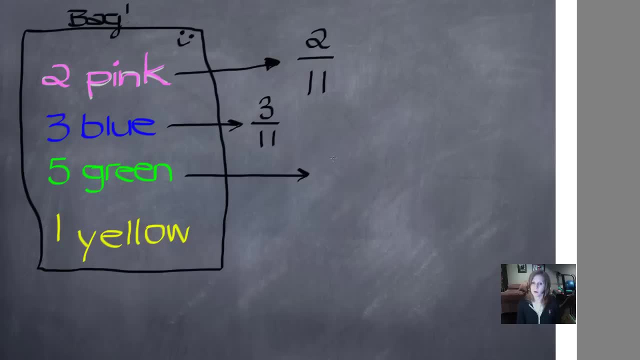 There are five green pieces of paper, So we would write five chances out of eleven that we would pull out a green piece of paper And there is one piece of yellow paper, So there's only one chance that we're going to pull out a yellow piece of paper. 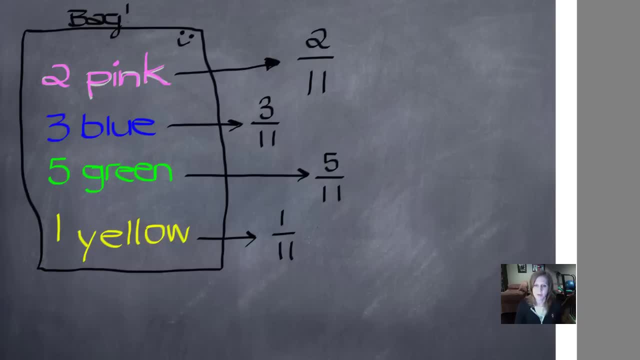 Now we're assuming that we're pulling out one at a time, So these are the fractions that represent the probability of pulling out each color of paper. One thing that you do need to know is that, since probability can be written as a fraction, 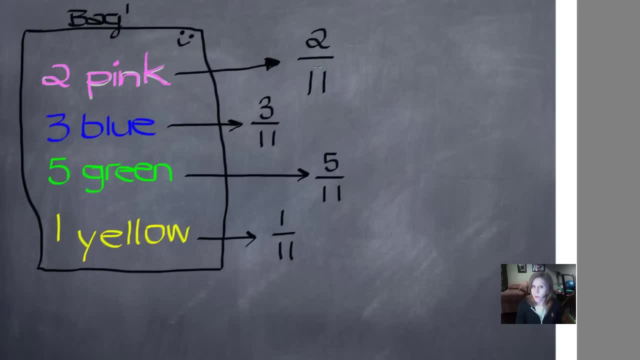 it is also simplified, always, because fractions are always simplified. So if we only had four green pieces of paper and ten was our denominator and we were trying to find the probability of pulling out a pink slip, two tenths because there are two pink slips. 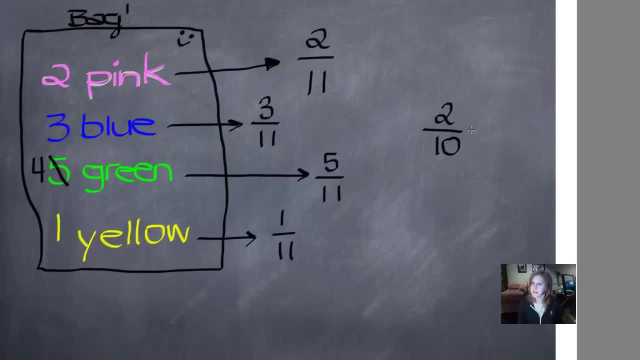 out of all the different colored pieces of paper. I would need to simplify this Now. remember, you can simplify by dividing by a common factor, or you can also make a cake, And so I'll come down here and write two tenths. 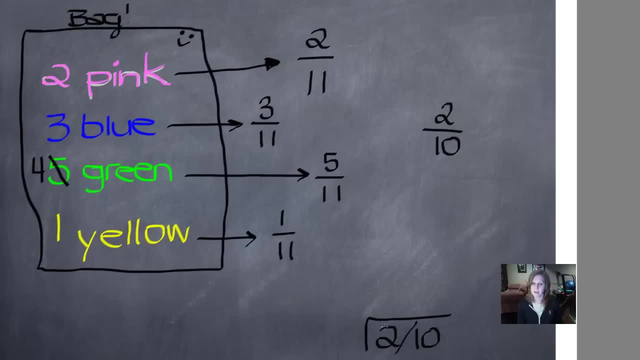 inside the bottom layer of my cake and ask myself what number divides evenly into both two and ten? And it's two. Two goes into two. one time Two goes into ten, five times. Next layer of my cake: What divides evenly into both one and five? 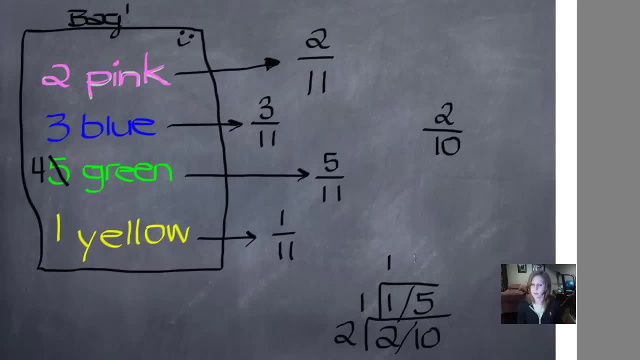 One is the only number. One goes into one one time. One goes into five, five times. Remember our saying: simplify, make a cake. look for the bride and groom. If this is our wedding cake, this is our bride and groom standing on top. 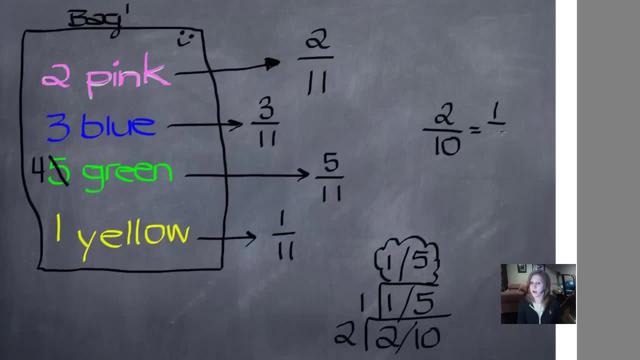 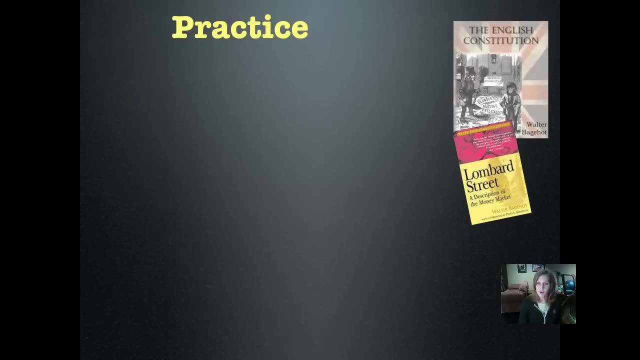 But we can't just leave it on top of the cake. We have to come over here and write it as an equivalent simplified fraction. Let's see if you can try some now. Here are your instructions for your practice problems. You're going to write the probability. 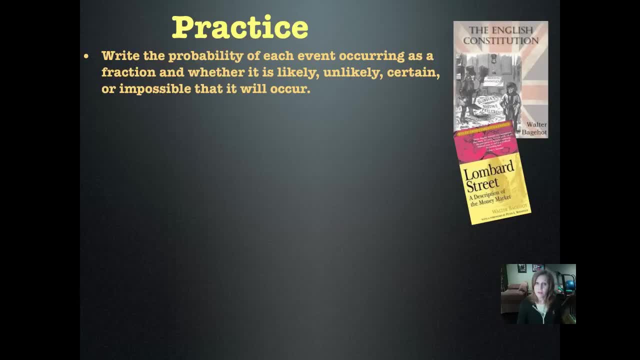 of each event occurring as a fraction and whether it is likely, unlikely, certain or impossible that it will occur. Remember, in order to be certain, it has to be the same number in the numerator as the denominator, because there are no chances that it won't happen. 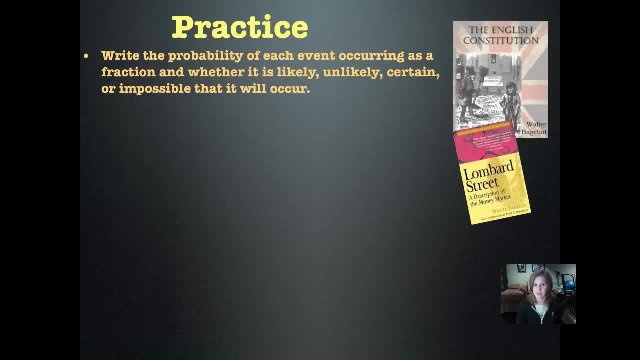 So for it to be certain to occur, you have to have one whole. basically, If it's impossible for it to occur, you would have a zero. You don't write a fraction as zero over however many choices you have or how many parts there are in all. 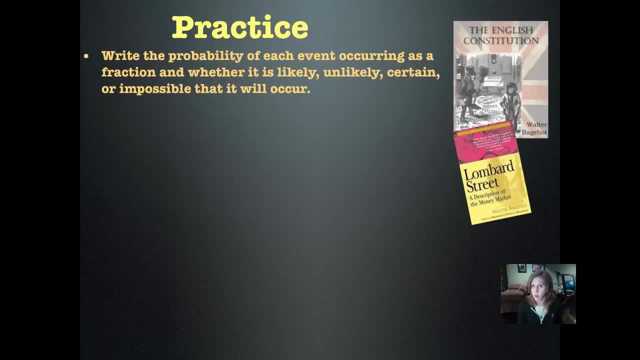 You just write zero, So certain would be represented by a one, Impossible would be represented by a zero, Likely would be represented by any fraction greater than one half, And unlikely would be represented by any fraction less than one half. Just for your information. 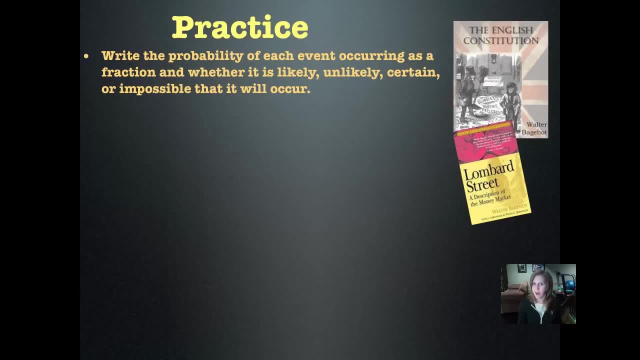 if your fraction is exactly equivalent to one half, that's called equally likely. You are just as likely for it to happen as for it not to happen. Let's try some. If Ruben puts the letters of his name in a bag, what is the probability that he will pull out the letter B? 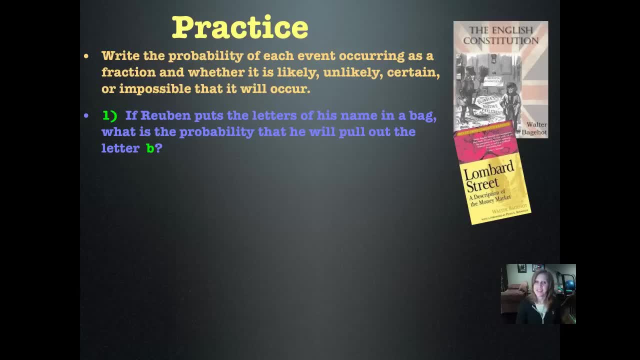 So write it as a fraction and then write whether it's likely, unlikely, certain or impossible that it will occur. Pause it and push play when you've written it down. Did you write one sixth and unlikely? I hope so, If you count all of the letters in Ruben's name. 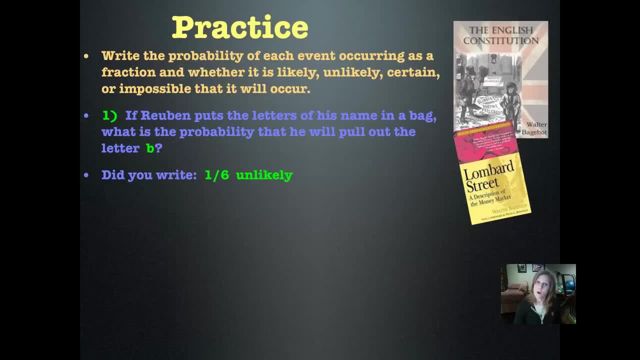 he has six letters in his name. There is only one B, So one is your numerator, That represents the B And the six represents all of the letters in his name. One sixth, One sixth isn't anywhere close to one half And if you need to check that, 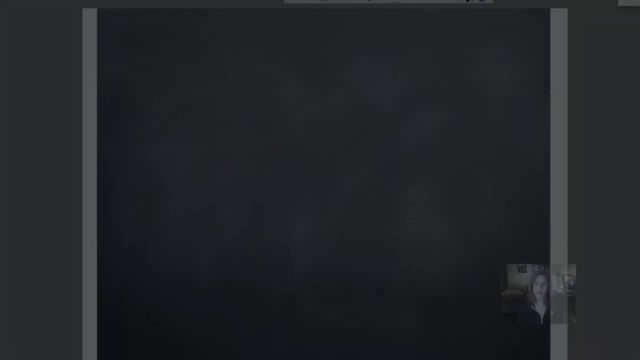 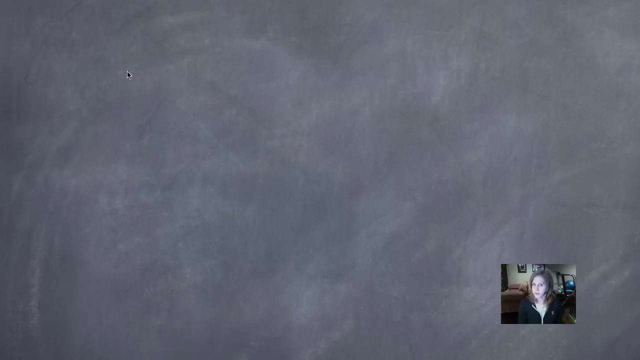 you can do. Well, let's look and see what we can do. I want to show you how you can compare it with one half. if you're not sure about the fraction- Although any time a fraction is equivalent to one half- you know that it can be simplified to one half. 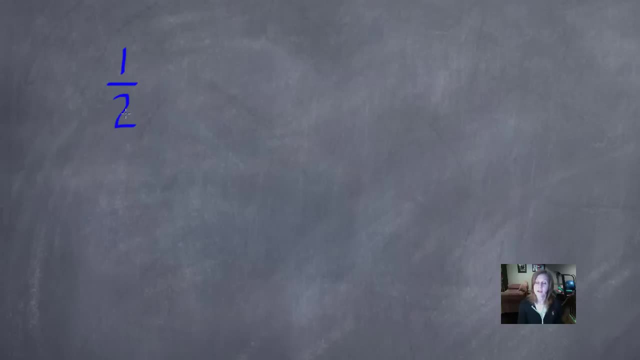 One half is a unit fraction because it has one in its numerator. Now if I end up with the fraction one sixth, and I want to know if it's greater than or less than one half, I just write one half next to it and cross multiply. 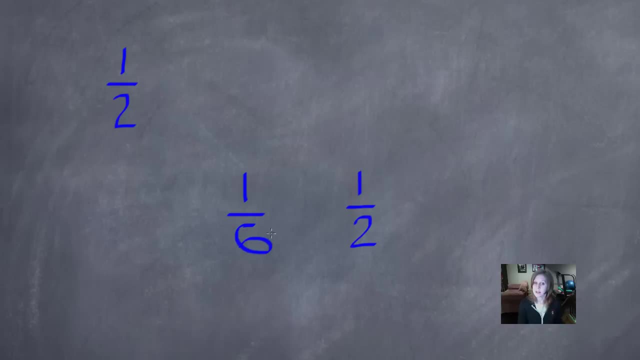 Starting at the lower denominator, six times one is six. Write it above it and circle it, And then start with your other denominator. two times one is two. Circle it Now. six is definitely greater than two, Or two is less than six. 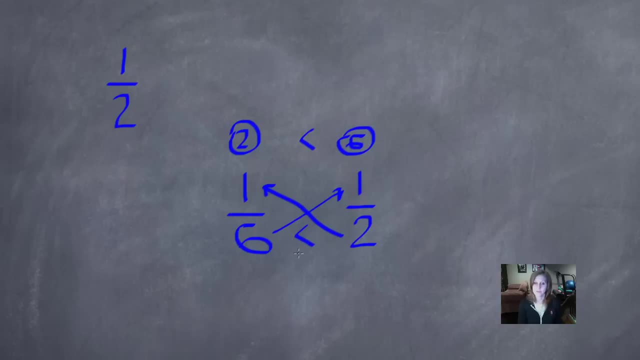 So one sixth is less than one half. So because we know it's less than one half, it's unlikely that it will happen. It's unlikely that we'll pull a B out of the bag that has letters of Ruben's name in it. 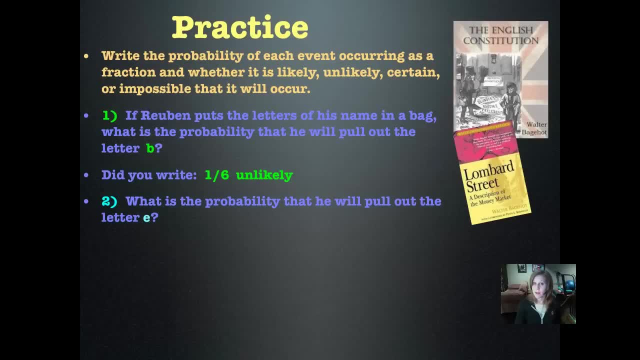 Number two: What is the probability that Ruben will pull out the letter E, Write it as a fraction and then write whether it's likely, unlikely, certain or impossible that it will occur. Pause it and push play when you've written it down. 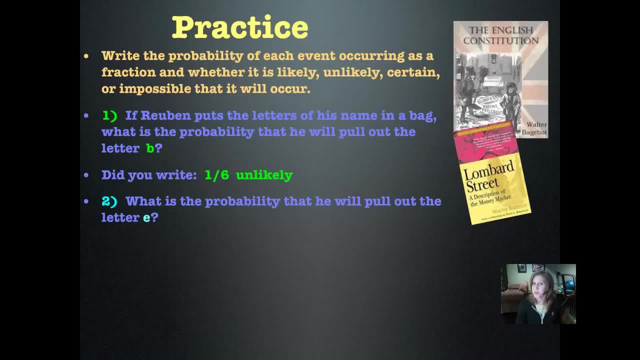 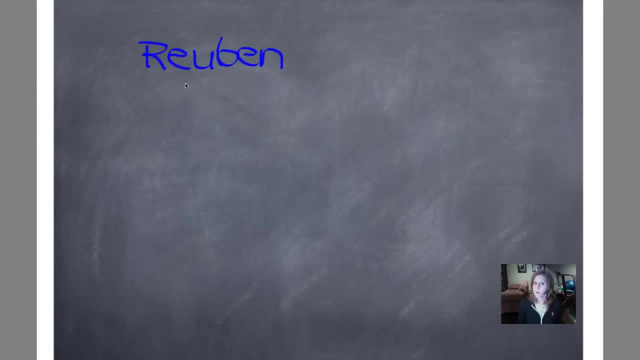 Remember you can always check your answer. Look back at the previous problem if you've forgotten how. So here are the letters in Ruben's name and we were asked to find the probability of him drawing out an E And we count how many letters we have in all. 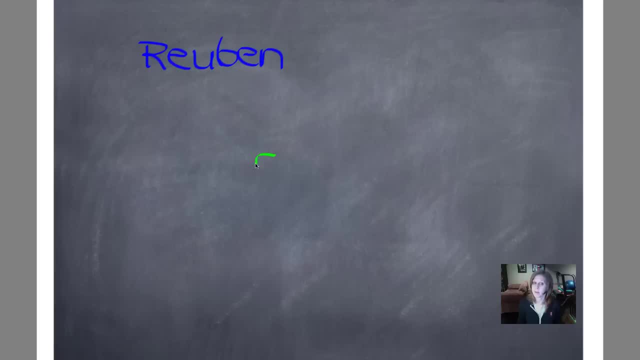 One, two, three, four, five, six. That's our denominator, how many we have in all, And then we count how many E's we have: One, two, There's one E, There's another E, Two, sixths. 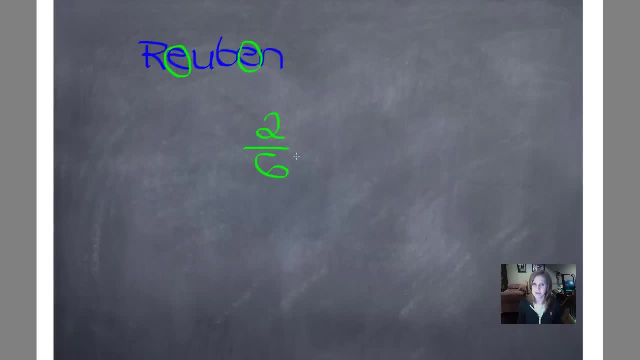 But remember, probability as a fraction needs to be simplified. So I'll come down here and make a cake. In the bottom layer of my cake I write my fraction and ask myself what divides evenly into two and six And two does. 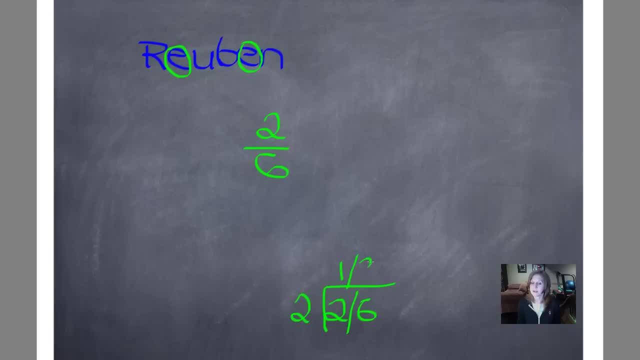 Two goes into two one time. Two goes into six three times. What goes into one and three, Just one. One goes into one one time. One goes into three three times. Remember, when you've repeated those two fractions, you're done. 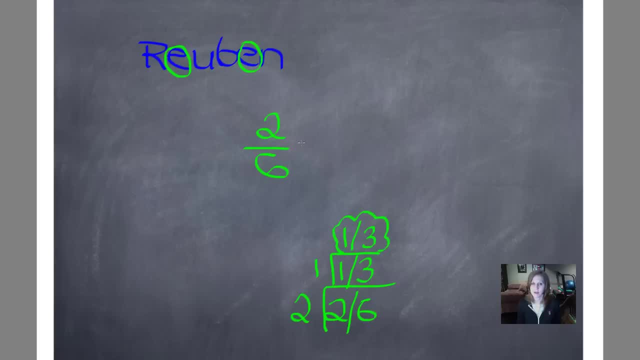 Look for the bride and groom. So two sixths is equivalent to one third, and that's in simplest form. We also call it reducing it to lowest terms. Now I'm not sure if one third is greater than or less than one half. 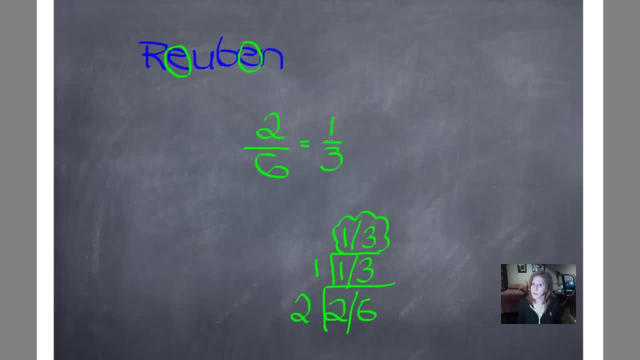 I know it's not three over three, which would equal one, so it's definitely not certain that he'll pull out an E. He might pull out a B or an R or a U or an N. It's also not impossible that he'll pull out an E. 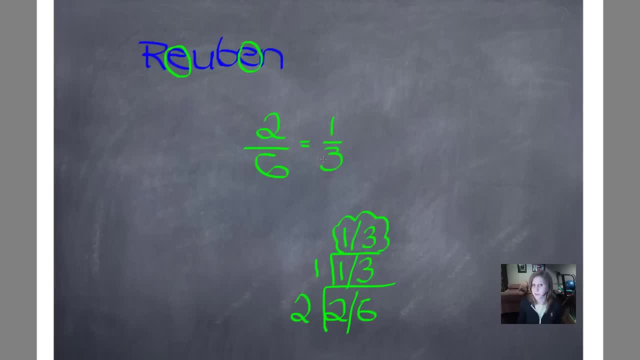 because it's not zero. He does have a chance of pulling out an E. There are E's in his name. If I asked you what is the probability of him pulling out a Q, That would be zero, so it would be impossible. 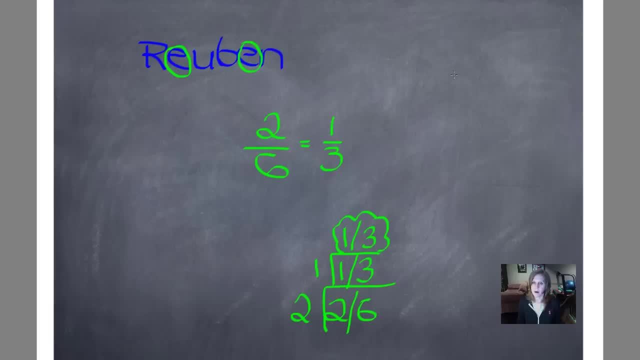 Now. so we're going to compare one third to one half by cross. multiplying Three times one is three and two times one is two. Hmm, Three is greater than two, so the fraction underneath the three is greater than the fraction underneath the two. 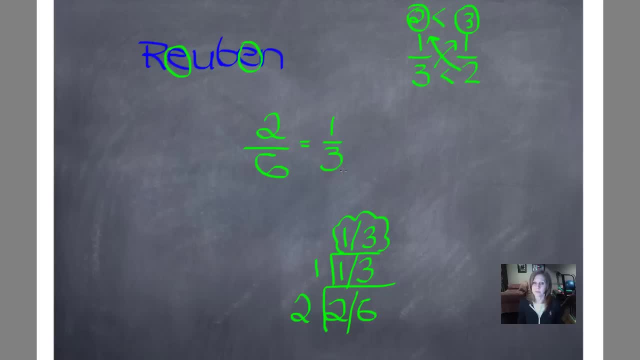 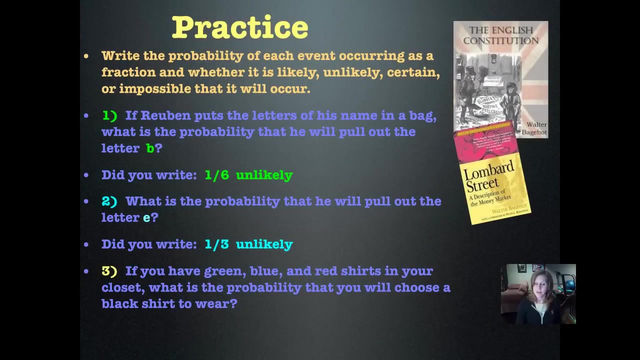 One half is greater than two. Two is greater than one third. So since one third is less than one half, we know it is unlikely that Ruben's going to pull an E out of the bag. Number three: If you have green, blue and red shirts in your closet. 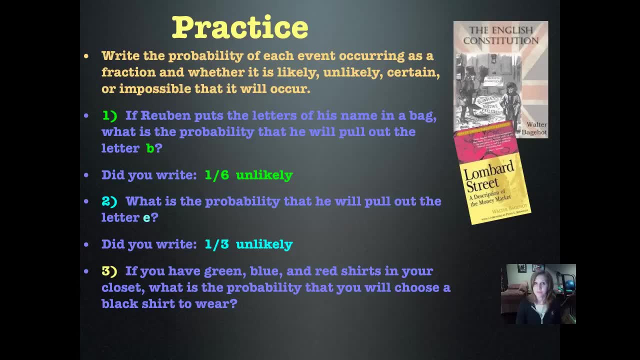 what is the probability that you will choose a black shirt to wear, Pause it and push play when you've written the fraction, and whether it's likely, unlikely, certain or impossible that it will occur, Pause it and push play when you're ready. when you're ready. 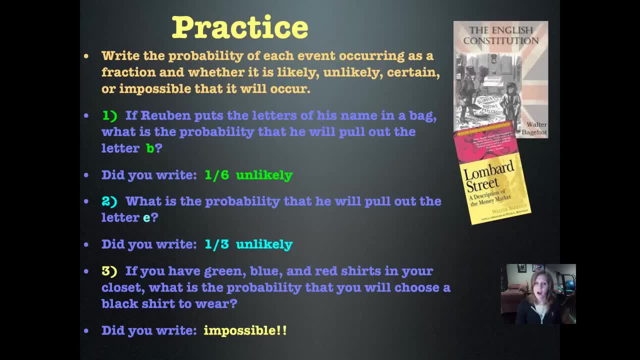 Did you write impossible? There are zero chances, not even written as a fraction. zero chances that you're going to pull a black shirt out of your closet if all the shirts in your closet are green, blue or red. No chance, And don't think about. 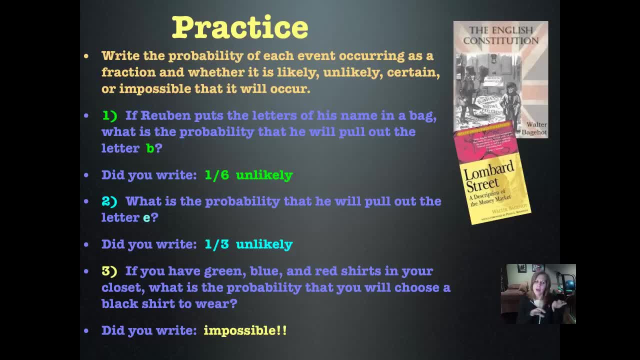 well, what if my little brother left that black shirt wadded up in the corner? Huh-uh, This is math land If I say there's only green, blue and red shirts in the closet. that's all the colors of shirts there are in the closet. 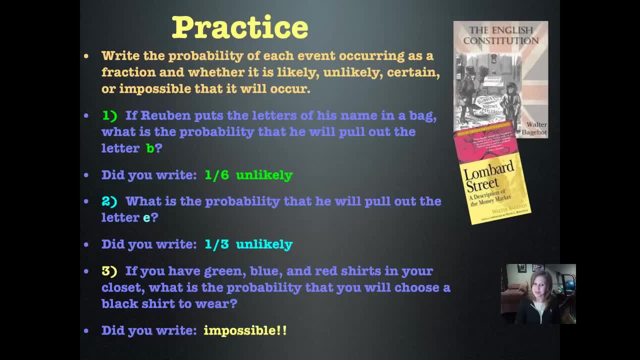 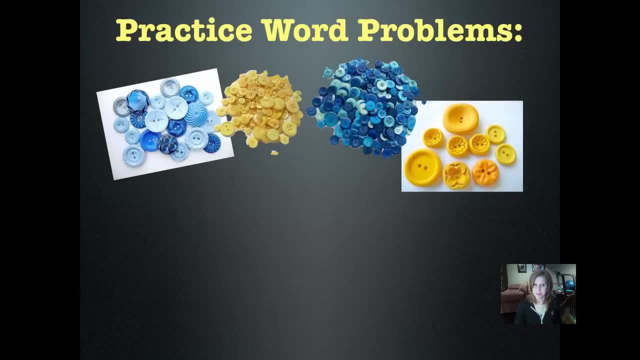 So you can say with certainty that it is impossible that you will wear a black shirt to school from that choice of shirts, It's time to practice word problems. I'll bet our word problem has something to do with buttons, If Cameron has eight yellow buttons. 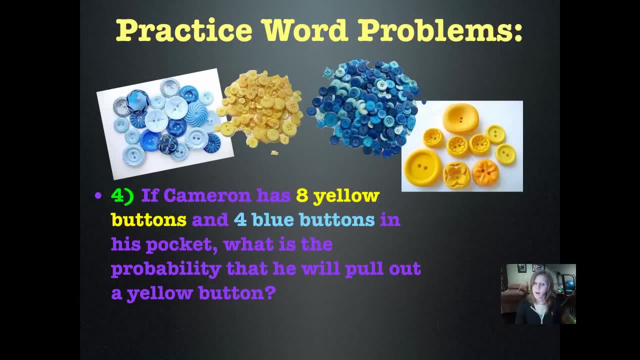 and four blue buttons in his pocket. what is the probability that he will pull out a yellow button? Write it as a fraction and then write whether it's likely, unlikely, certain or impossible. Pause it and push play when you've got it. 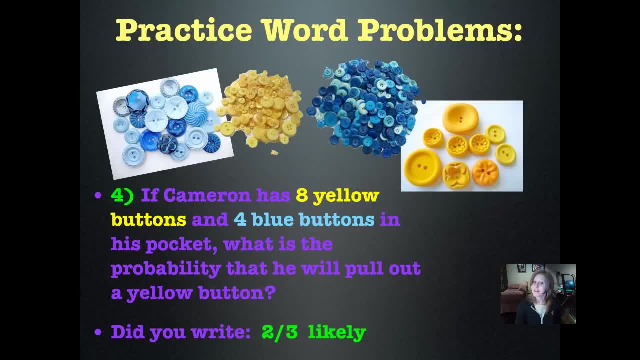 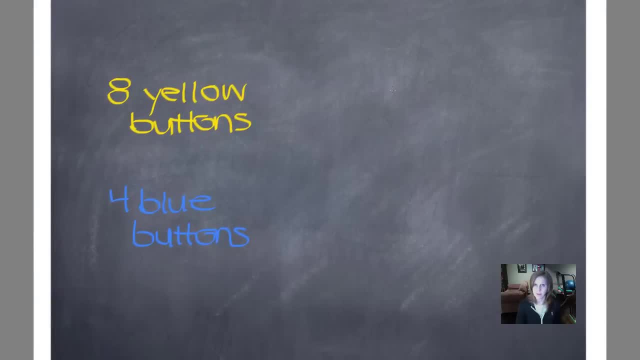 Did you write two-thirds? It's likely. Let's see how we did that. The first thing we need to do to write probability as a fraction is to find out how many buttons we have in all in his pocket. So we add eight plus four. 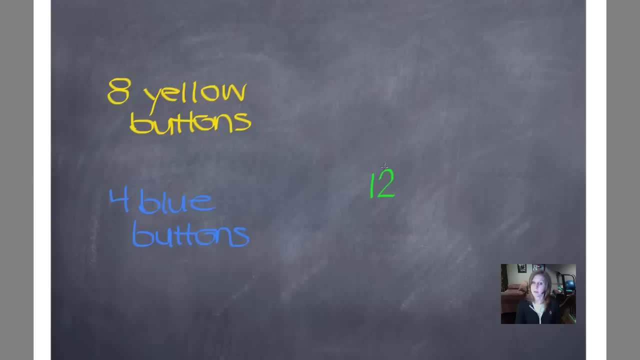 and we get twelve. Twelve is our denominator. Then we write down how many yellow buttons there are. There are eight, So there are eight chances that he will pull out a yellow button. Eight-twelfths is the probability of pulling out a yellow button. 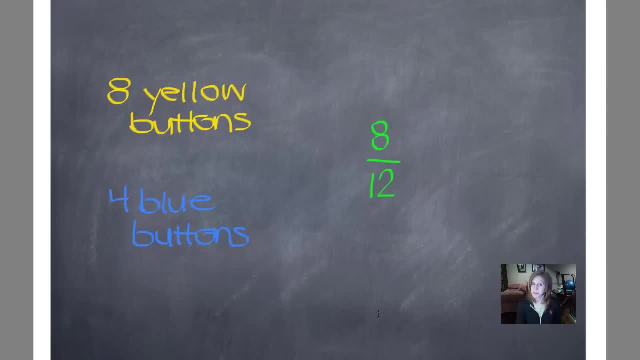 But eight-twelfths isn't simplified. They're both even numbers. So let's put eight-twelfths in our cake in the bottom layer. What divides evenly into eight and twelve, Let's go with two. Two goes into eight four times. 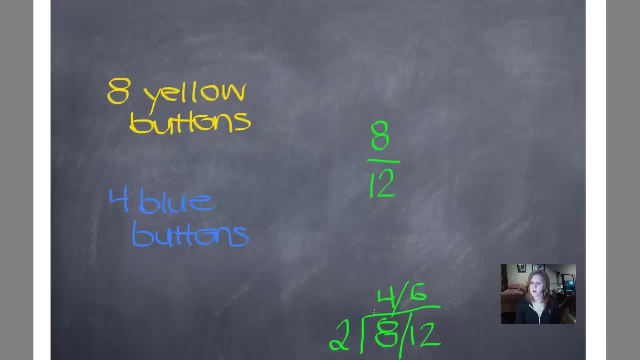 Two goes into twelve six times. What divides evenly into four and six, Two. Two goes into four two times Two goes into six three times What divides evenly into two and three, Just one. One goes into two two times One goes into three, three times. 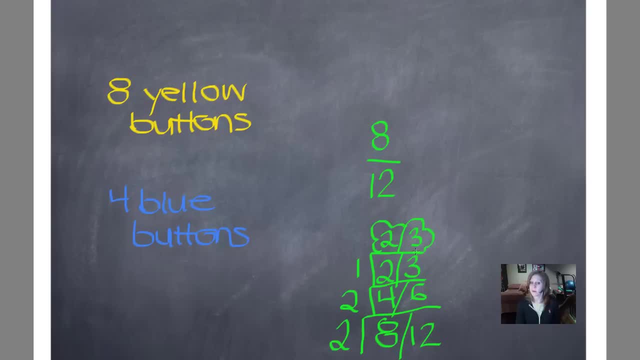 Simplify: Make a cake, Look for the bride and groom on top. So eight-twelfths is equivalent to two-thirds. Two-thirds is the probability that he will pull out a yellow button, But we want to know if it's likely or unlikely. 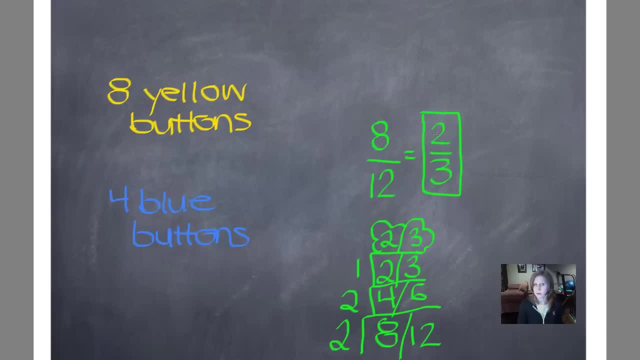 We know it's not certain because our fraction isn't three-thirds or twelve-twelfths, which would equal one, And we know it's not impossible because our answer isn't zero. There are yellow buttons in his pocket, So we're going to compare.